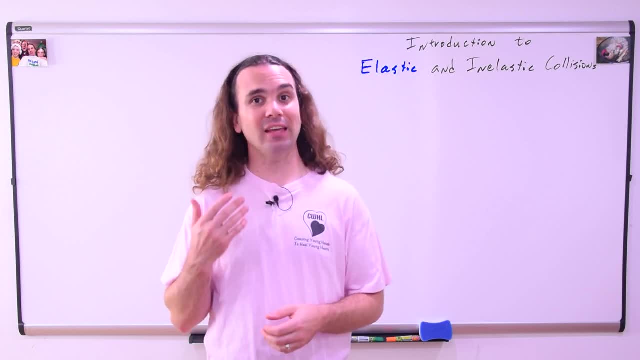 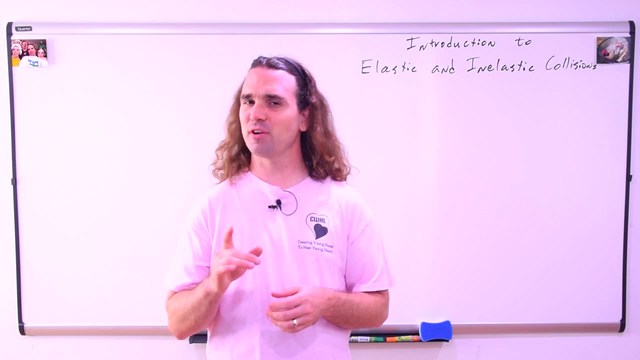 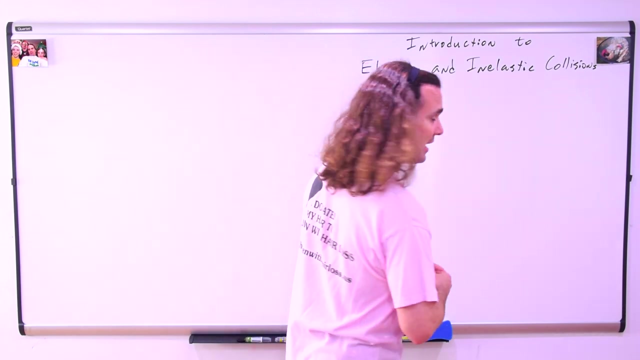 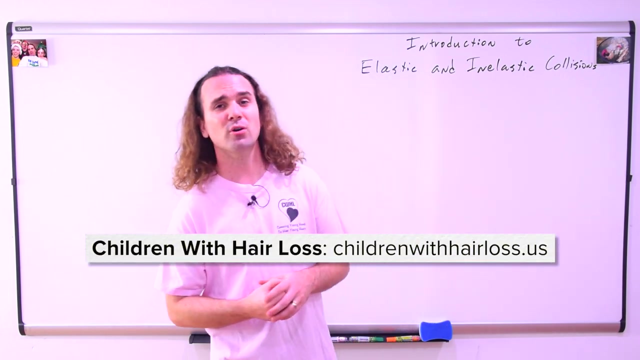 Mr, Good morning. Let's define elastic and inelastic collisions- Flippin' Physics, Mr. But first it is Charity Day of our Spirit Week. Charity Day, Mr. My charity is Children with Hair Loss, a non-profit organization which provides human hair replacements to over 300 children per year at no cost. 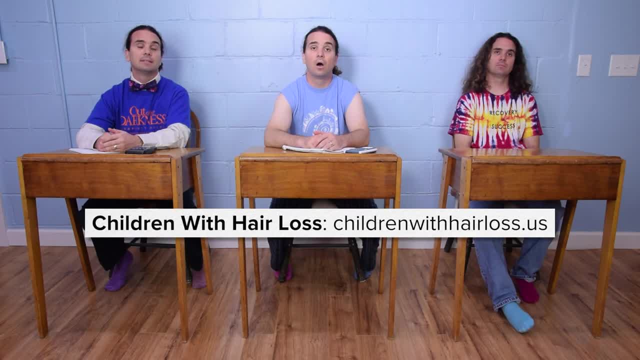 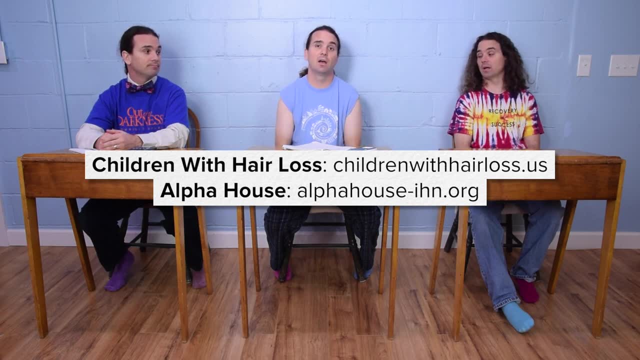 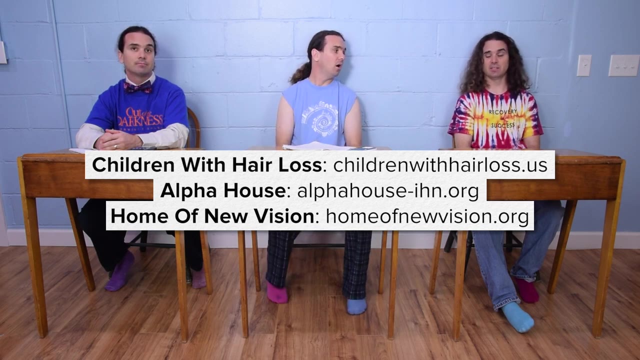 Gentlemen, what are your charities? I'm representing Alpha House. It's a homeless shelter for children and their families. My t-shirt is from Home of New Vision, a non-profit dedicated to help people affected by the disease of addiction. Recovery equals success. 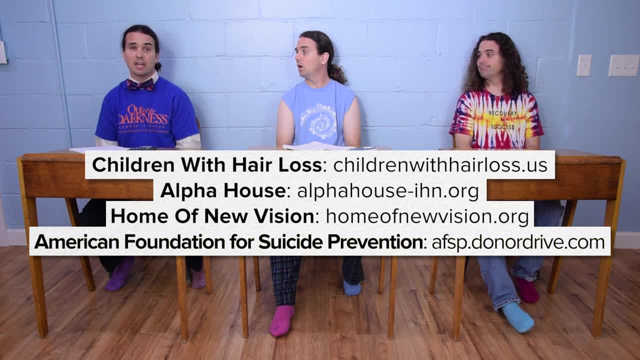 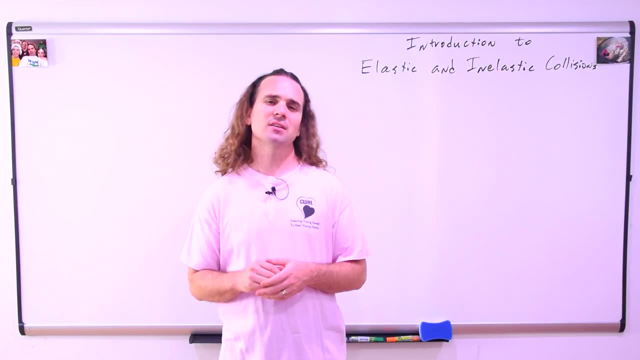 And I'm here for the American Foundation for Suicide Prevention and their Out of Darkness Community Walks to support survivors of suicide loss. Gentlemen, those are all worthy causes. Thank you very much. Alright, back to the physics. Let's start with something called an elastic collision. 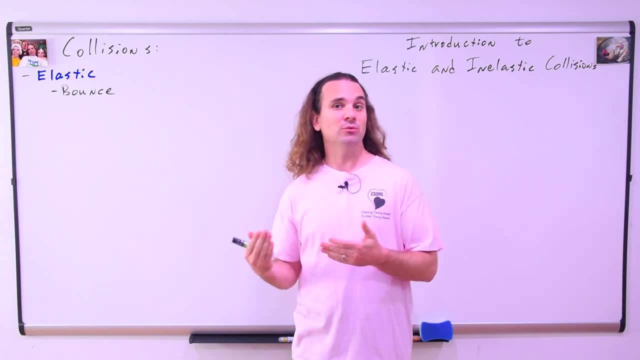 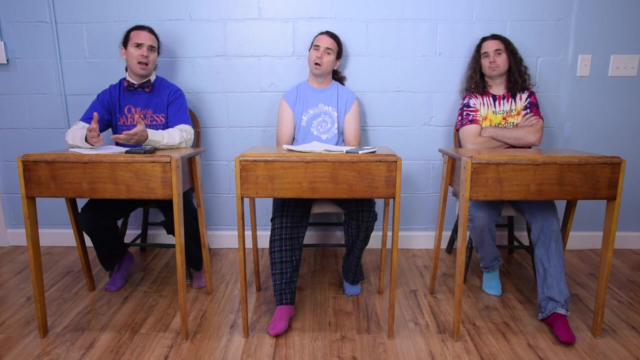 In an elastic collision, the objects bounce off of one another. Billy, is momentum conserved in an elastic collision where the two objects bounce off of one another? Is momentum conserved in an elastic collision? I'm sorry, but how should I know? 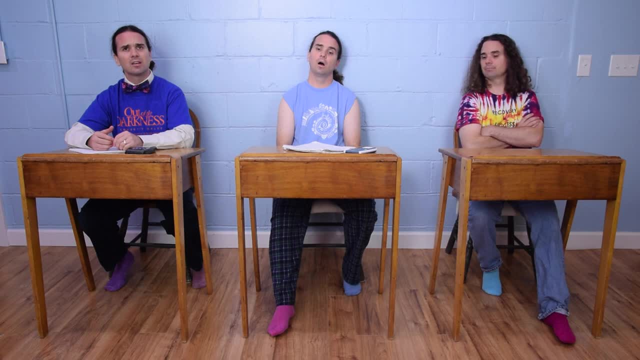 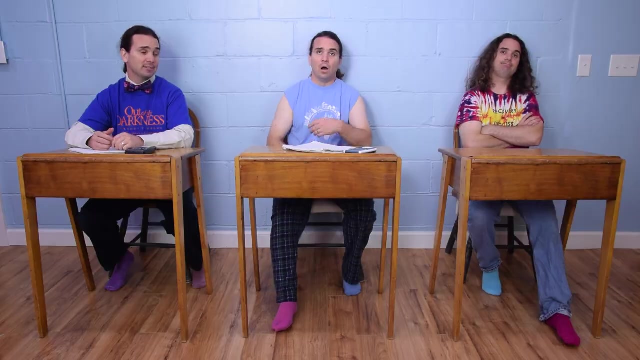 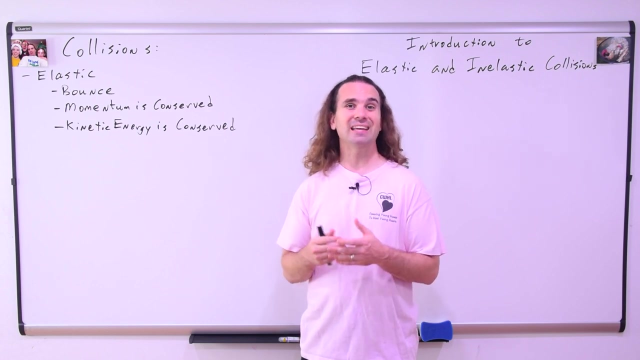 You should know, because the answer is actually built into the question. An elastic collision is a collision, And momentum is conserved during all collisions and explosions. Right, Therefore, momentum is conserved during an elastic collision. Thanks, In addition to momentum being conserved, kinetic energy is also conserved during elastic collisions. 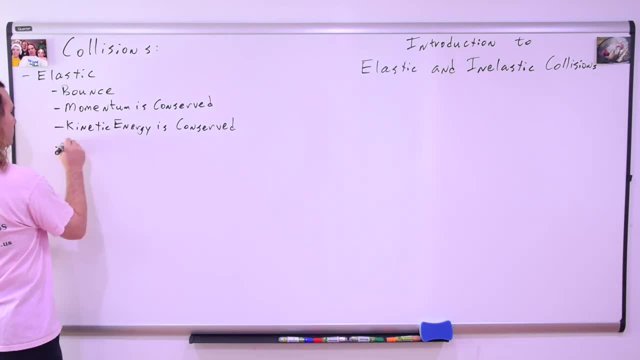 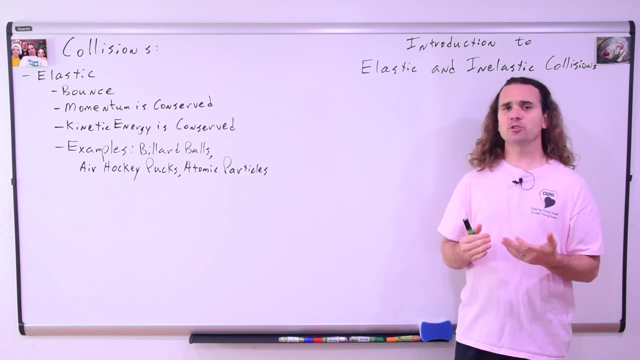 Some examples of elastic collisions are Collisions between billiard balls, collisions between air hockey pucks and collisions between atomic particles are all examples of elastic collisions. Now let's talk about inelastic collisions. Class is momentum conserved in inelastic collisions. 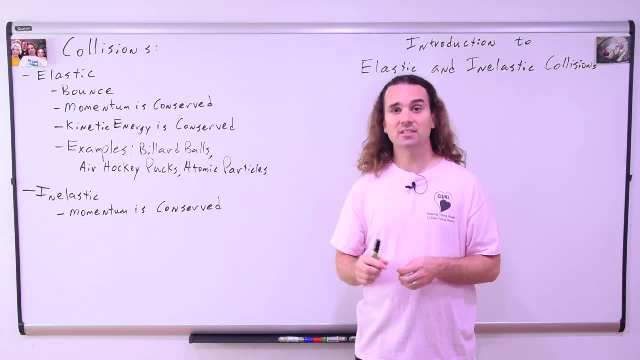 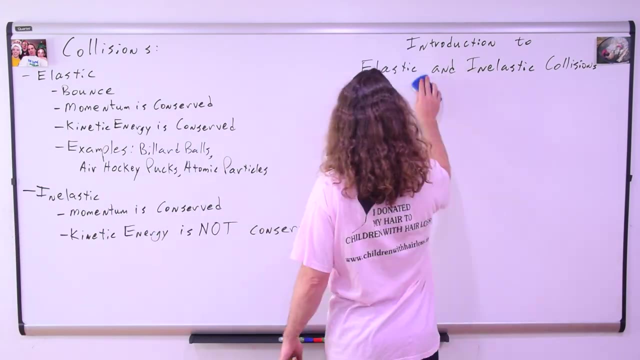 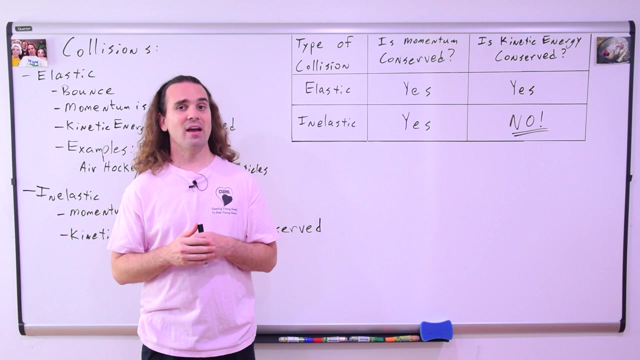 Yes, it's a collision. What sets an inelastic collision apart from an elastic collision is that kinetic energy is not conserved during an inelastic collision. Let's make a table with this information. Realize, we now have the words elastic and inelastic, which can sound very similar to one another. 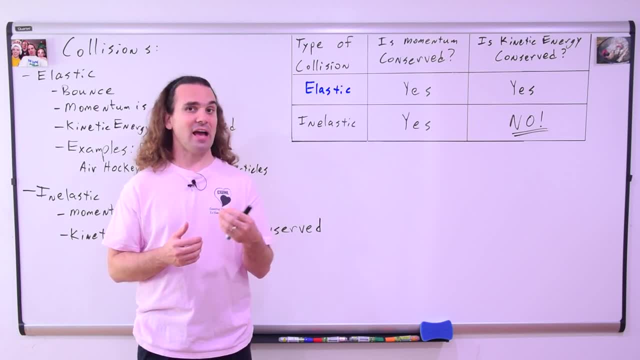 Especially when you say something like: In an elastic collision, kinetic energy is conserved. However, in an inelastic collision, kinetic energy is not conserved. So please be very careful to carefully enunciate the words elastic and inelastic. I will. 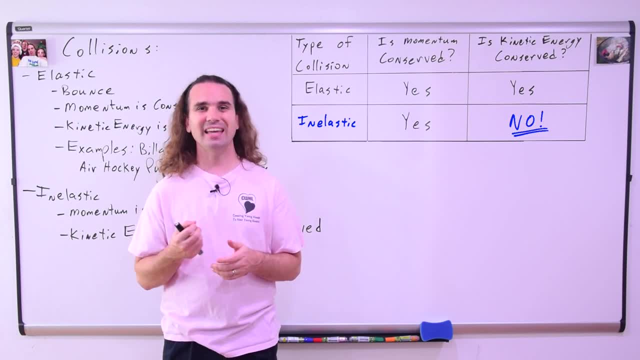 The reason kinetic energy is not conserved during inelastic collisions is because during inelastic collisions the objects deform and that change in shape of the object heats up the object. In other words, the deformation of the object causes the kinetic energy to be converted into thermal energy. 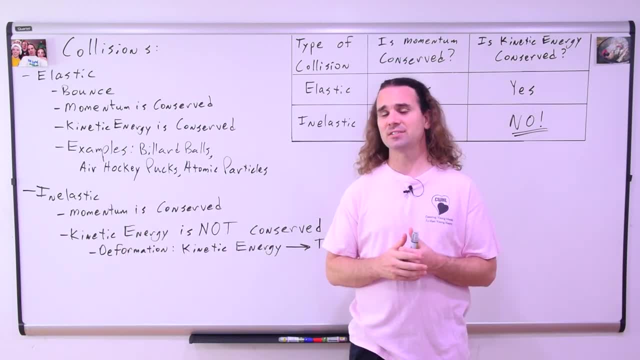 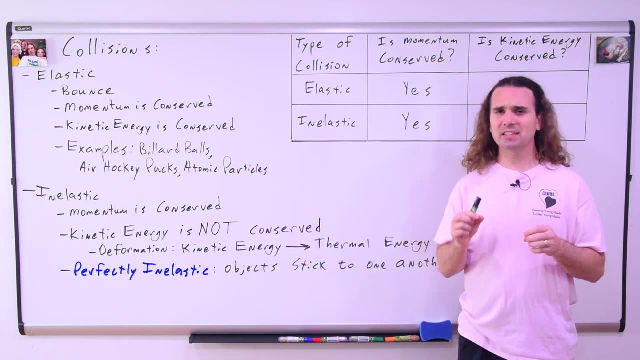 I will point out that there is also a specific type of inelastic collision, which is called a perfectly inelastic collision. A perfectly inelastic collision is where the objects run into and stick to one another. Sometimes you'll also hear a perfectly inelastic collision. 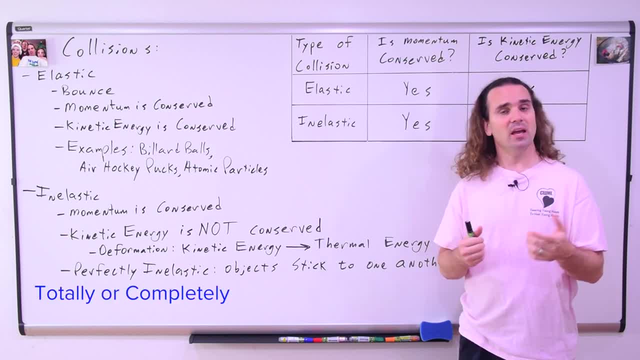 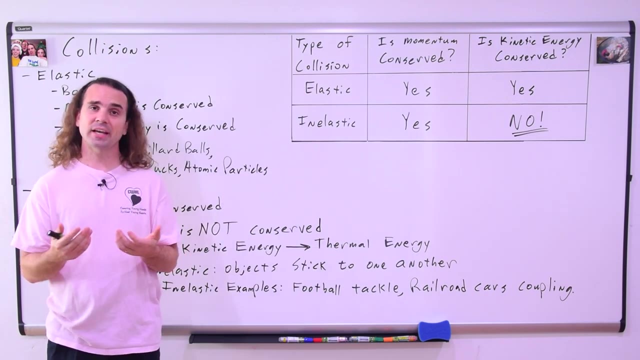 referred to as a totally or a completely inelastic collision. However, I prefer the term perfectly inelastic collision. So some examples of perfectly inelastic collisions are two football players colliding and holding onto one another or a tackle, or two railroad cars running into one another and coupling. 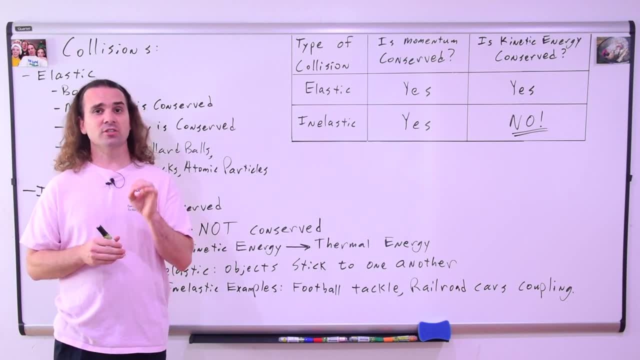 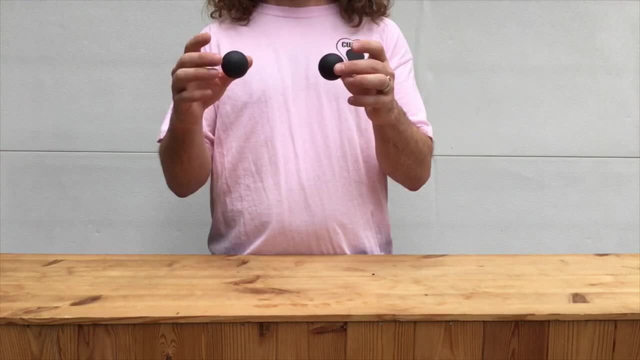 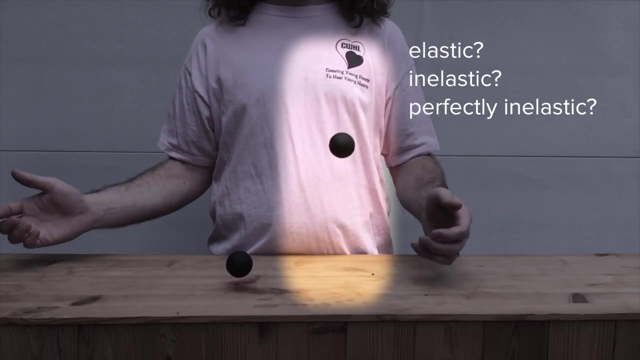 Okay, so now let's take a look at a demonstration of some collisions. When I drop these two balls from the same height, the one on your right bounces much higher than the one on your left. Bo. is the collision on your right an elastic, inelastic? 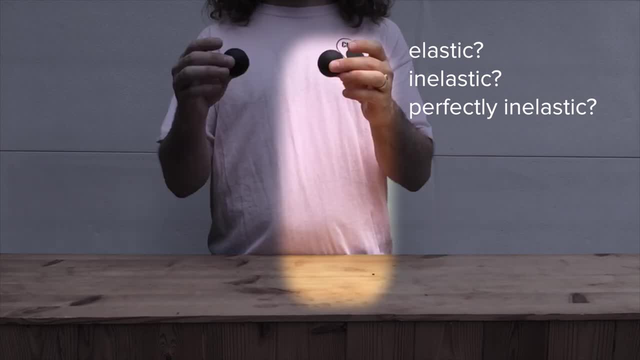 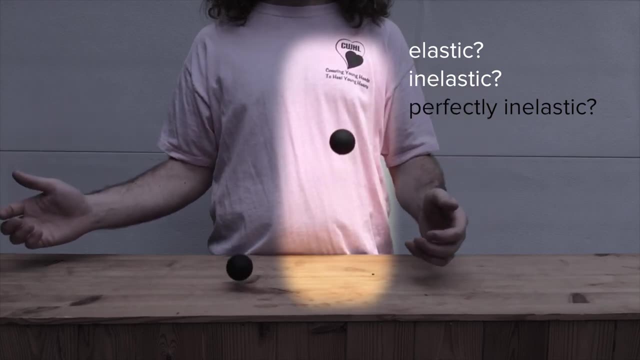 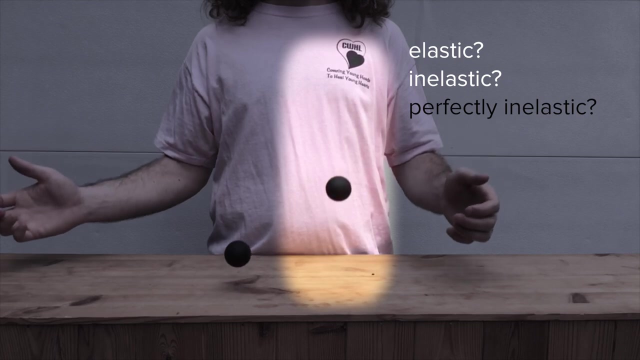 or perfectly inelastic collision. Well, I know it's not a perfectly inelastic collision, because the ball does not stick to the table. So is it elastic or inelastic? That's the question. In other words, is kinetic energy conserved or not?